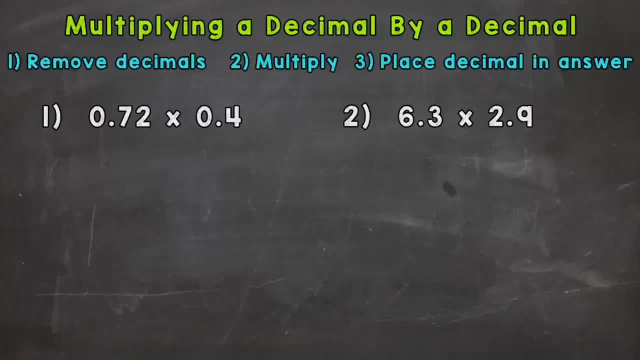 screen. And step one: we remove or forget about any decimals and we rewrite the problem. So we can rewrite it as 72 times 4.. Now these decimals will come back into play later in the problem. Step two: we multiply just like we would any other whole numbers. So 72 times 4 here, 4 times 2 is 8.. 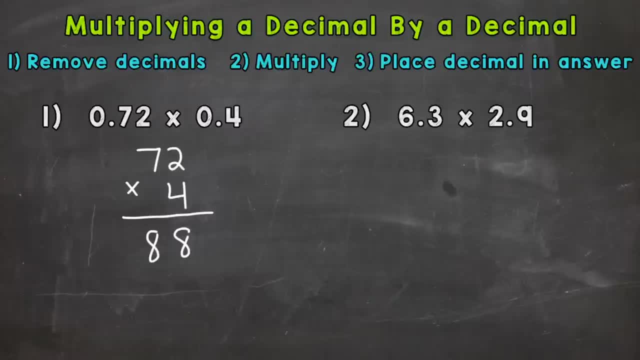 And then 4 times 7 is 28.. And we get 288 there. That brings us to step three, where we need to place the decimal correctly in our answer. So we go back up to our original problem and see how many digits are to the right or are behind a. 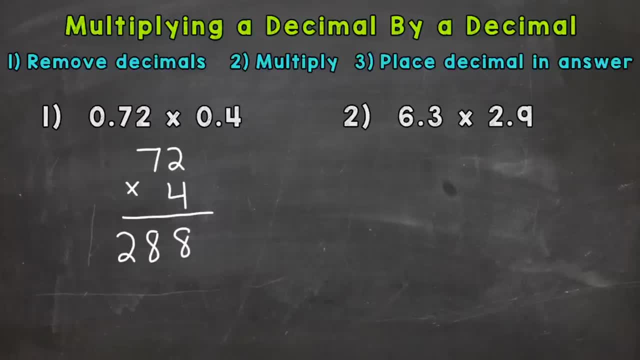 decimal, However you want to think of it. So we have this 7 here. This is 1,, 2, and 3.. I like circling them That way I don't forget anything. So that's 7,, the 2, and the 4 are all to the right. 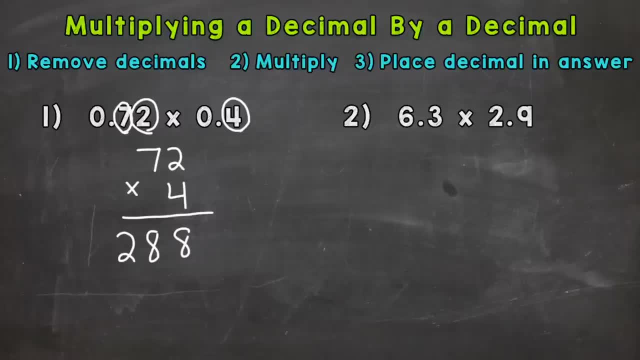 of a decimal. That means our answer needs to have three digits to the right or behind the decimal. So we can do one of two things With a whole number. the decimal comes at the end here And we can think of it like this: Moving it in 1,, 2,, 3.. And placing the decimal here And we get an answer of. 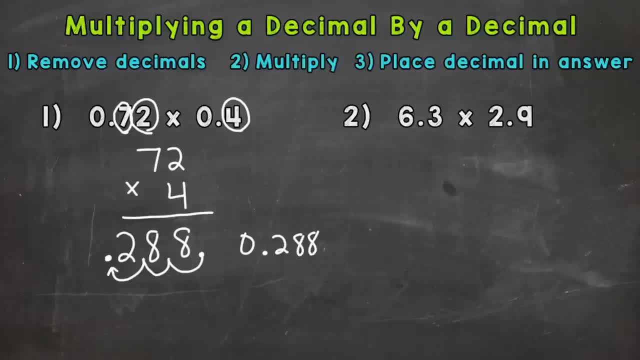 288 thousandths, which is correct. Or we can take a look at- I'm going to rewrite 288: here We have 288 thousandths And we can just place the decimal there. So a couple different ways of thinking, of placing that decimal correctly. They both will give you the same answer. So our final answer is: 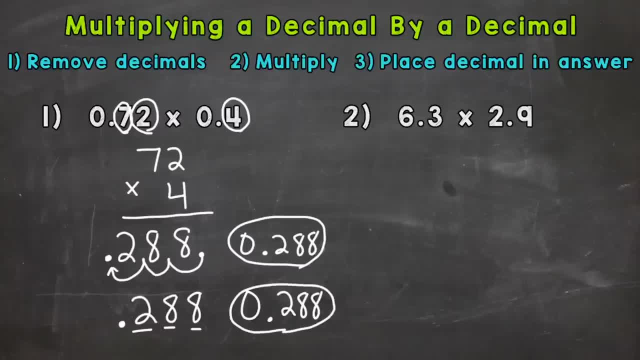 288 thousandths. On to number two, where we have 6 and 3 tenths times 2 and 9 tenths. So first step: remove and forget about any decimals And we end up with 63 times 29.. Now we multiply.